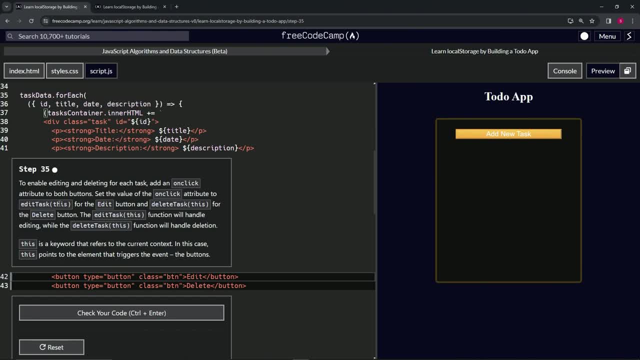 the value of the on-click attribute to edit task. this, with this is the argument. and then for the edit button. pardon me, and that's going to be for the edit button and delete task. this for the delete button. The edit task: this function will handle editing, while the delete task- this function. 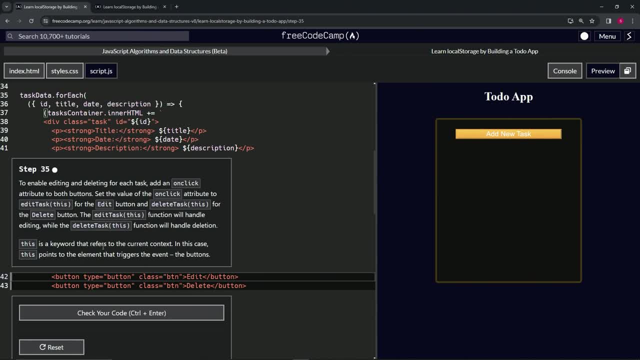 will handle deletion. This is a keyword that refers to the current context. In this case, this points to the element that triggers the event, AKA the buttons. All right, So this one's a hilarious one. Uh, we'll go. we'll go into the. 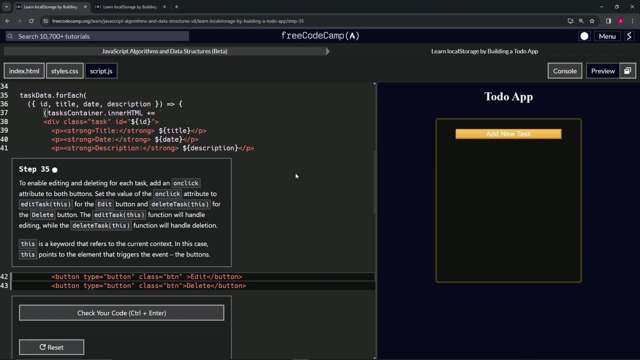 hilarity in just a second. Let's, let's get through this first. So we'll say, uh, on-click equals, and then we'll do the um quotes like that. inside of the quotes We'll do uh, edit. 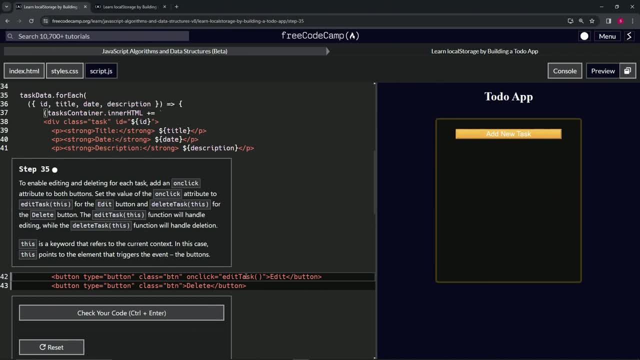 task And then we'll say inside of these parentheses: this like that, right. So now let's take from this closing angle bracket all the way to the uh closing quote on button on BTN. copy that and drop it off right after the closing quote on this. on a deletes BTN. 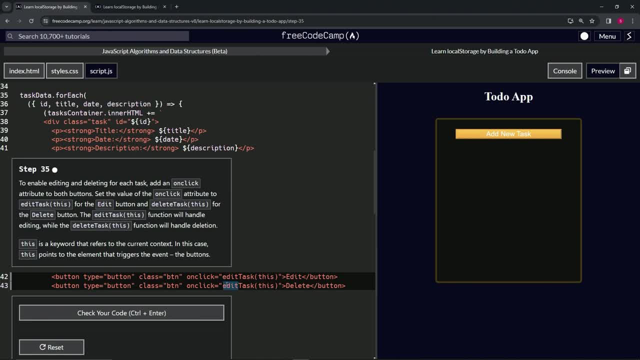 And then let's change edit to delete. All right, Delete. So if you're anything like me, you're probably saying: huh, what's this, What's that? Yeah, You know, Uh, and then you go through and you say: wait, we haven't, we haven't made anything. 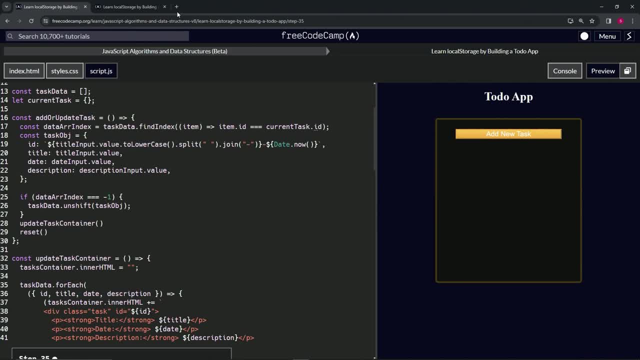 like this. And then you go and say, okay, on-click attribute, uh, blah, blah, blah, blah blah in Google, And then you can't find anything. Well, you know what? This is one of those classic. 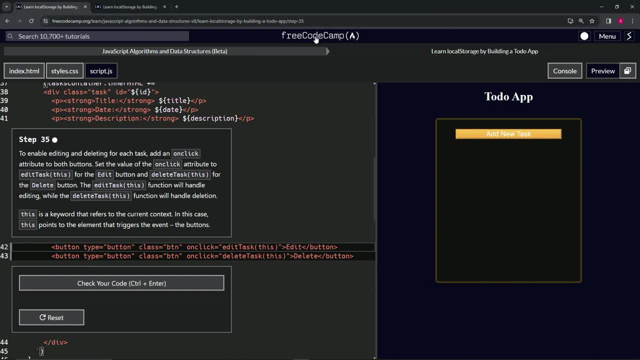 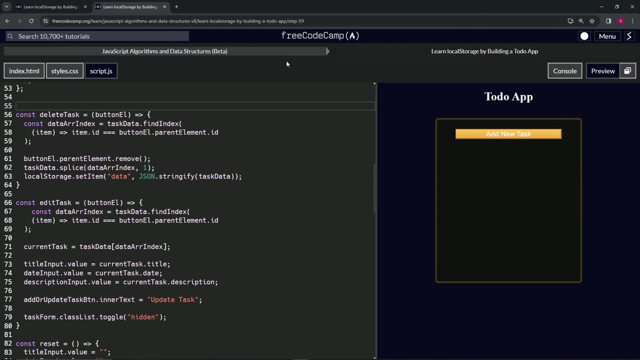 those classic, uh, those classic moves by free code camp. In fact, the thing is, we just haven't made these functions yet. So we're declaring, we're, uh, doing function calls for functions We haven't declared. And to prove that, here's step 59.. And wouldn't you know, at some point we're going to make both.